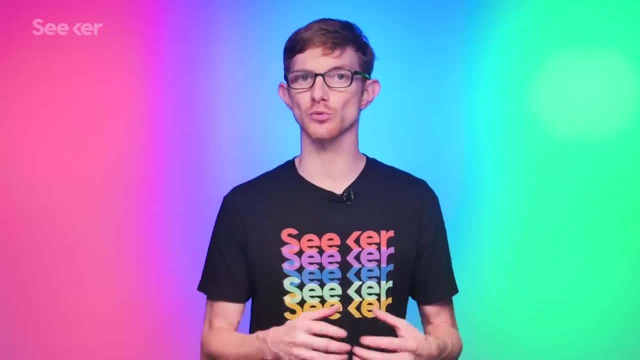 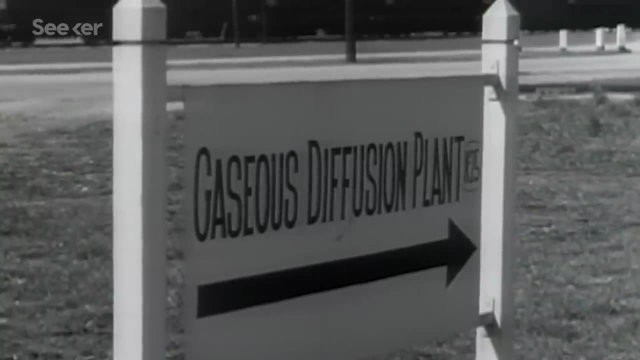 That's where enrichment comes in. A couple of approaches have been used to enrich uranium. The one used by the Manhattan Project to build the first atomic weapons was gaseous diffusion. In order to separate the uranium isotopes, the first step was to turn it into a gas. 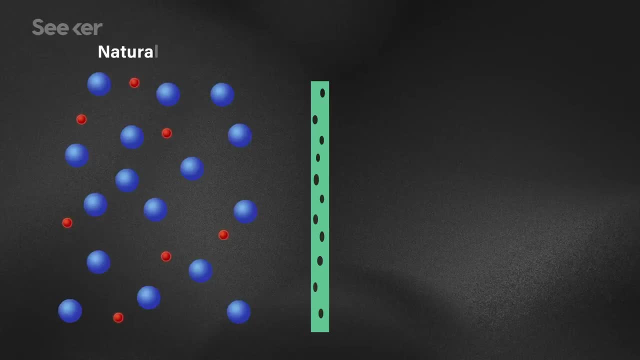 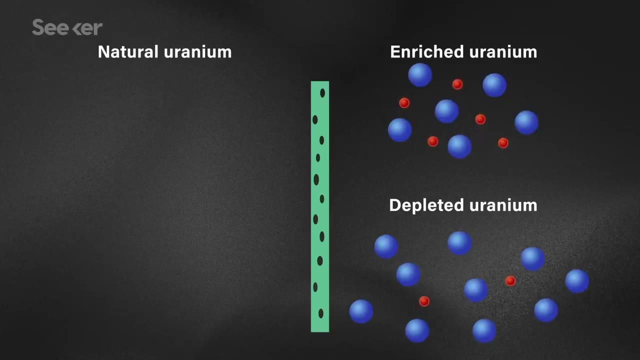 By adding 6 fluorine atoms. Once gaseous, the uranium hexafluoride was pushed through membranes whose holes were just big enough to let the molecules through. The lighter U-235 moves slightly more quickly through the barriers. So after several hundred membranes, 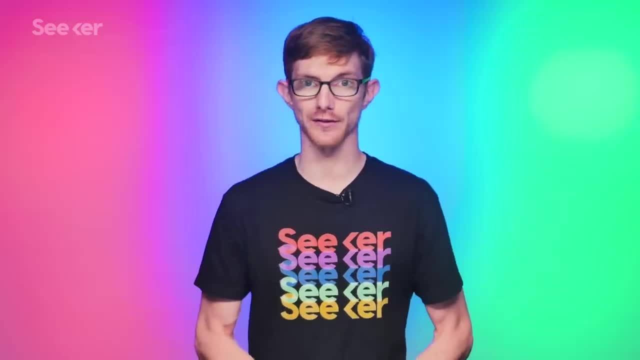 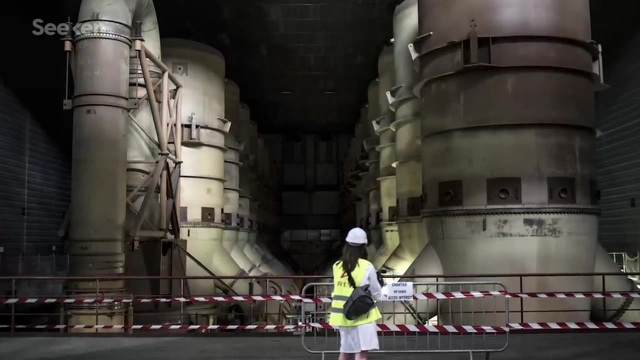 the gas at the other end had the required amount of U-235.. The more modern method is using centrifuges, which are cylinders that spin at very high speeds enough to separate the lighter U-235 from U-238.. The first step is the same, but 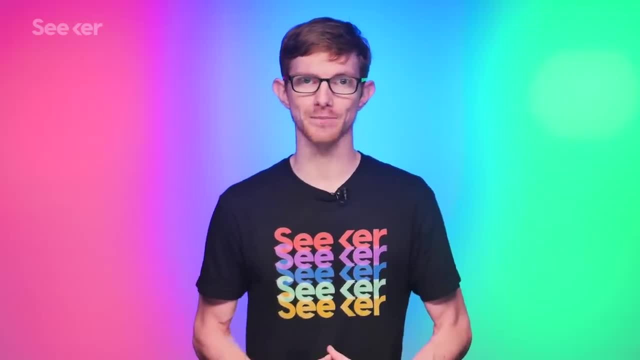 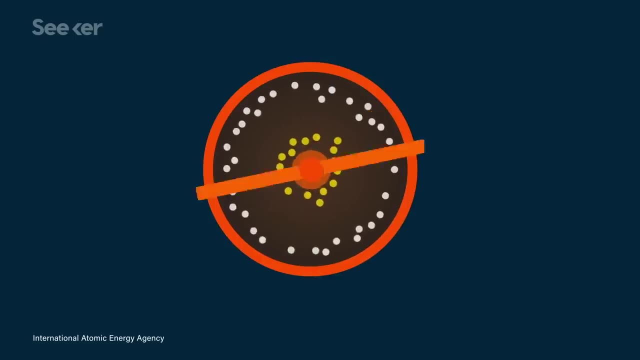 turning all the uranium into gaseous uranium hexafluoride. Then, like a hipster with a vinyl collection, get spinning. As the gas is spun around, the heavier U-238 will move towards the outside of the cylinder, while the U-235 will drift to the center. The slightly enriched 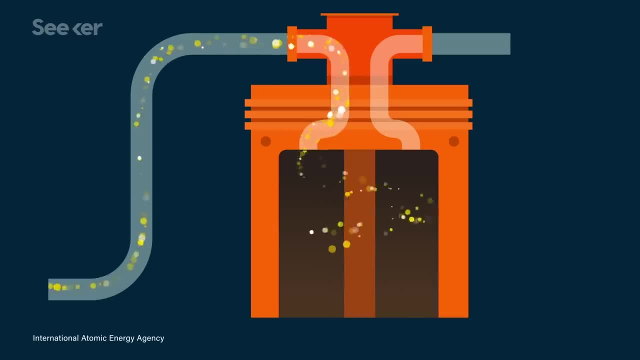 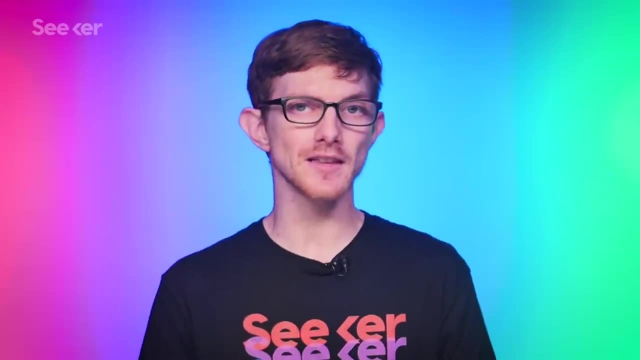 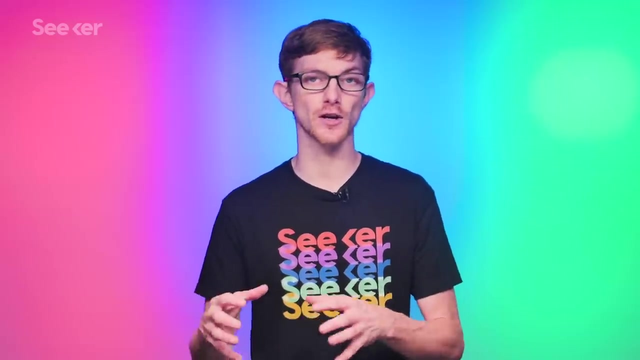 gas there will be piped out and fed into another centrifuge, And on and on it goes, using thousands of centrifuges connected in series and parallel formation, steadily upping the amount of U-235 in the mix enriched. it's a simple matter of rearranging the centrifuges to create weapons-grade uranium. 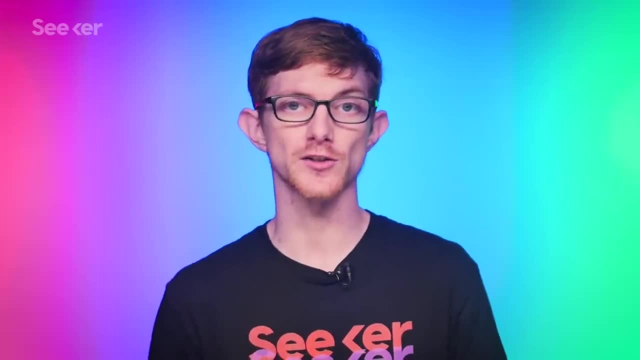 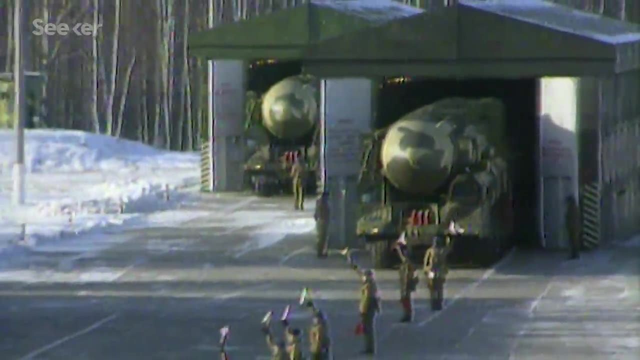 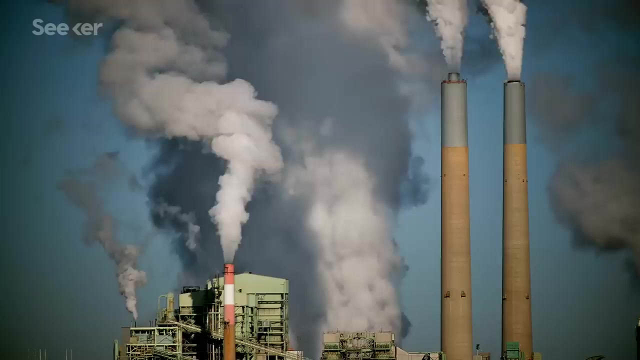 very quickly. That's why a vital part of ensuring a country is only using their nuclear program for peaceful purposes is inspecting how their centrifuges are arranged. The proliferation of nuclear weapons remains one of the most serious threats to the world, but nuclear power's potential to provide energy without adding greenhouse gases to. 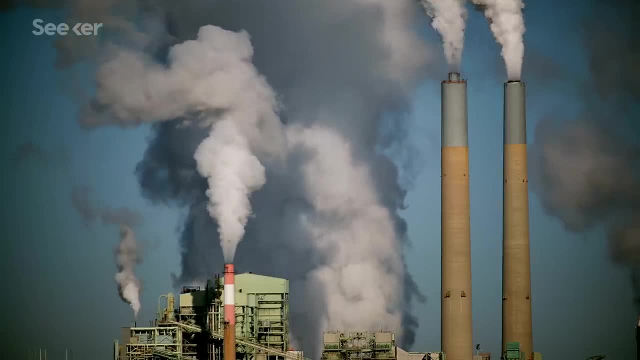 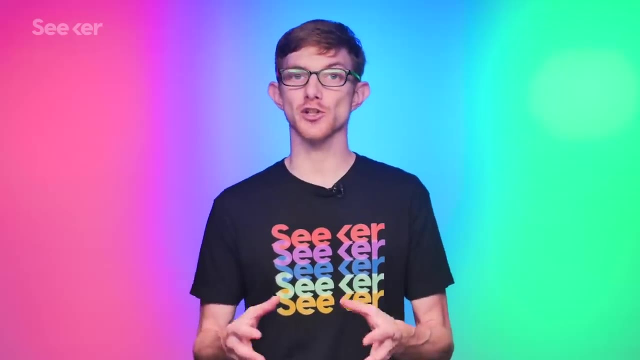 our atmosphere is a huge possible benefit for humanity. If we're going to use uranium for the good of us and the planet, then it just needs a little enrichment. While the centrifuges enrich uranium, they're also feeding the more concentrated U-238, the 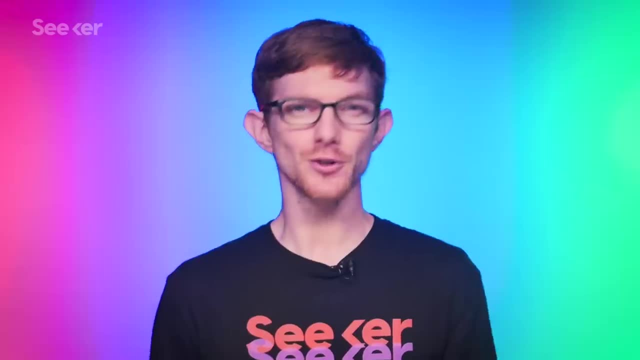 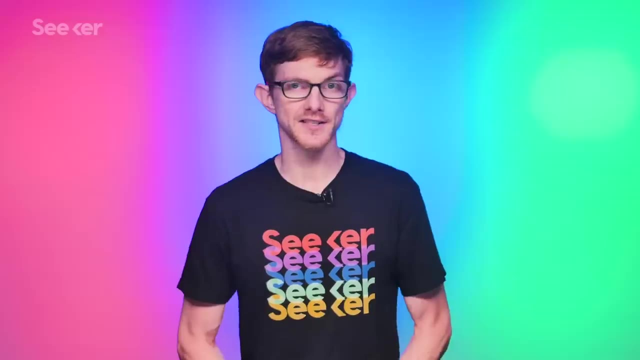 opposite direction, producing depleted uranium at the other end. Nuclear power is still something that worries a lot of people, and recently Russia decided to turn a boat into a floating power plant. To see if this is a bad idea, check out my video on it here. 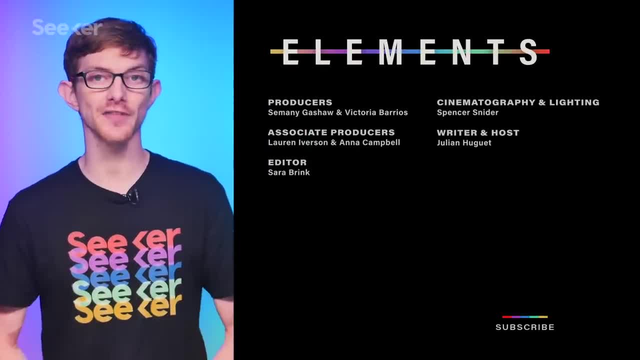 If you liked this video, let us know in the comments below. Make sure to subscribe to Seeker and thanks for watching. I'll see you in the next one.